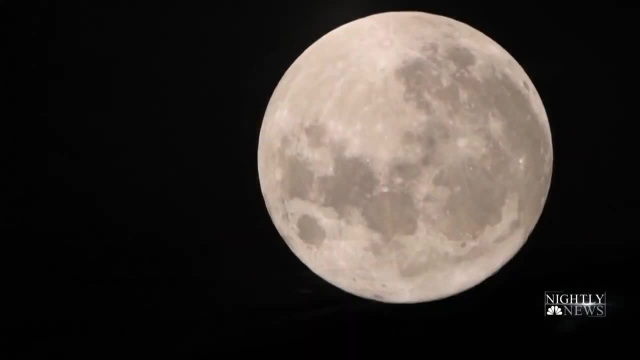 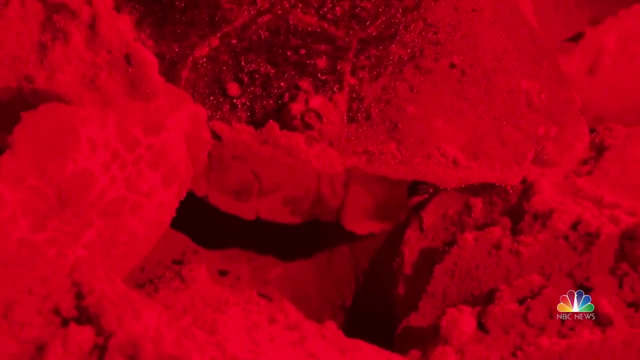 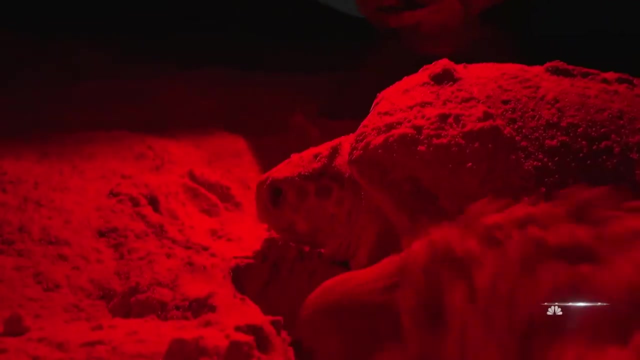 Early this morning, under the light of the supermoon, a loggerhead turtle, 30 feet from water's edge, begins to lay her eggs. This is always pretty fantastic. Fantastic, say biologists, because 20 years ago sea turtle nests were in steep decline. But this year, from beaches in 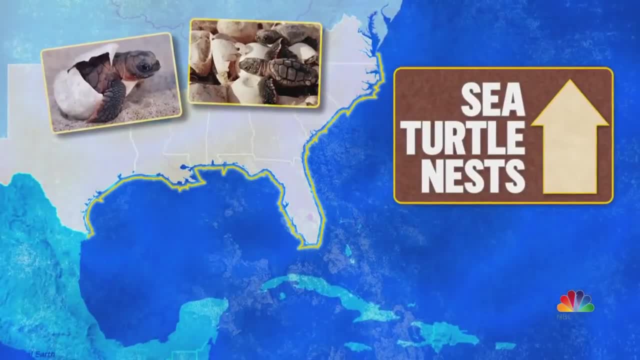 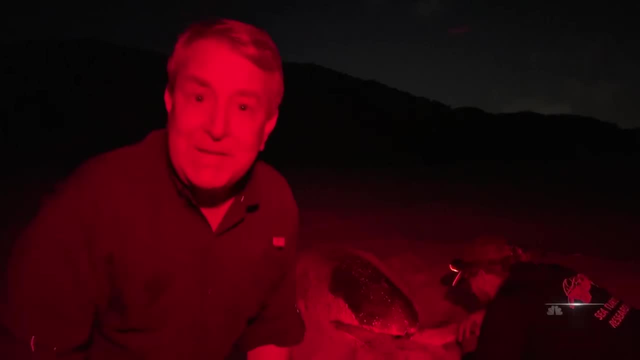 Virginia's south and all along the Gulf Coast a strong resurgence. It's been a prolific year and just 13 miles along Florida's east coast, more than 20,000 nests. But there are problems and it has everything to do with global climate change. A turtle's sex is determined not by 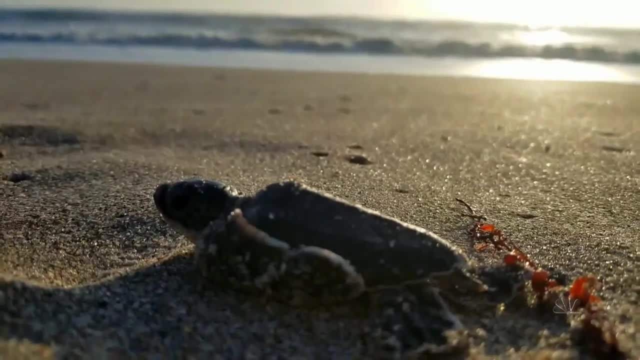 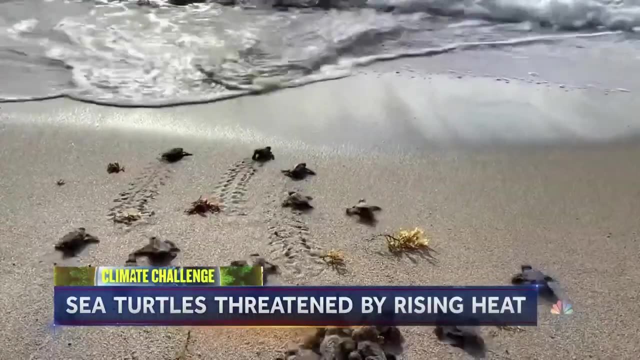 chromosomes. Rather, it's all about the temperature of the sand. There's an old saying in the sea turtle community: hot chicks, cool dudes, because you tend to end up with more females at warmer temperatures and more male hatchlings at cooler temperatures. Researchers say those hatchlings 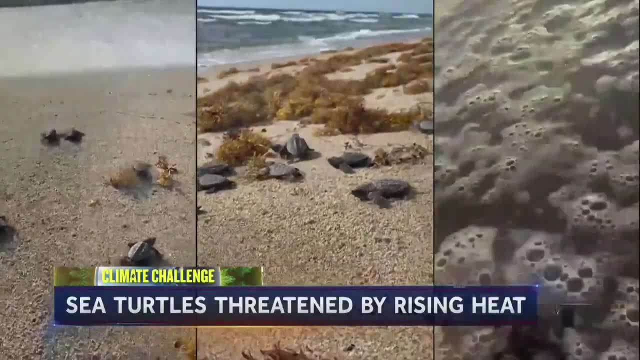 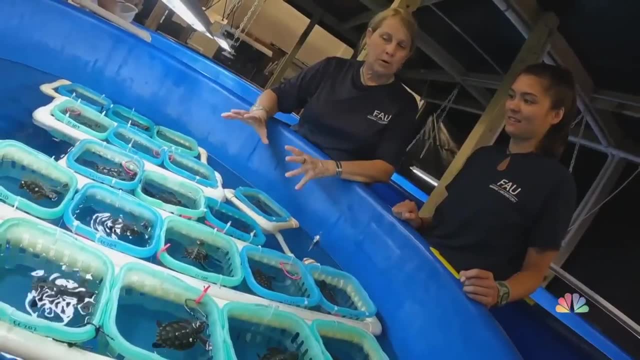 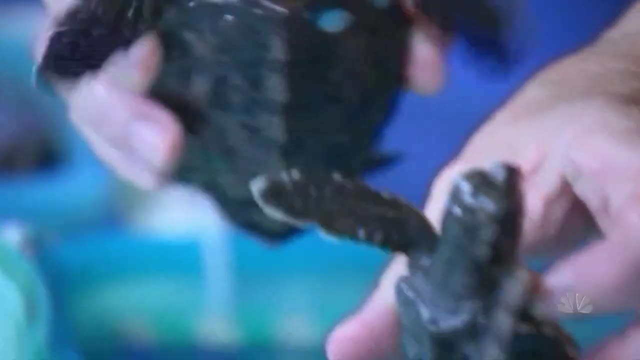 this morning were the most common. They're most certainly all female. We have this high percentage of all female years. Florida Atlantic University professor Jeanette Weineken says 82 degrees or below you get boys, 88 degrees or above girls. That's the problem, because you have to have boys, Plain and simple. 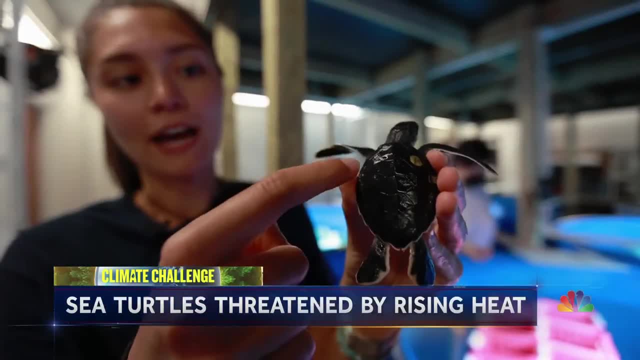 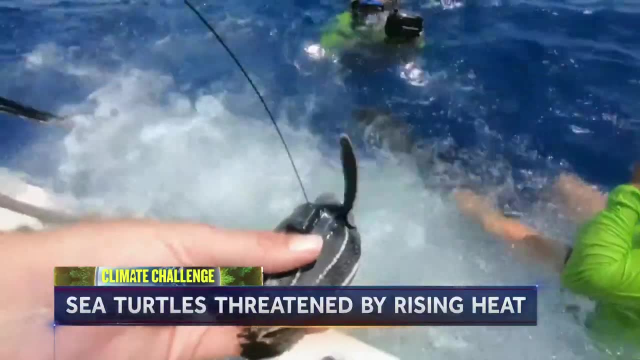 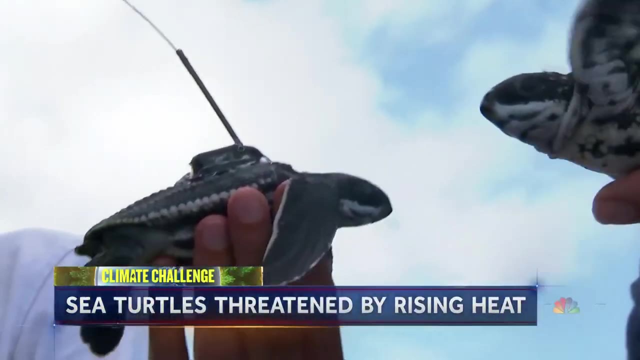 This is a loggerhead turtle. This is a green sea turtle. Those turtles threaten species 15 miles from shore, far from predators lurking on the beach, scientists with the most endangered of all turtles, the leatherback, With tiny trackers scientists hope to beat the odds. Currently, only one in a. 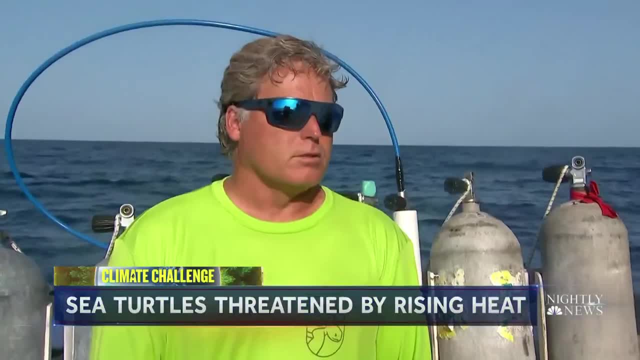 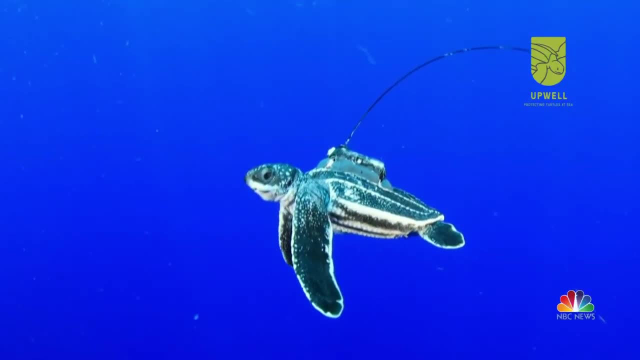 thousand makes it to adulthood. As leatherbacks go, so too do the oceans, and the oceans that we humanity depend upon. So their fate there is inextricably linked with our own. Kerry Sanders. NBC News- Melbourne Florida.